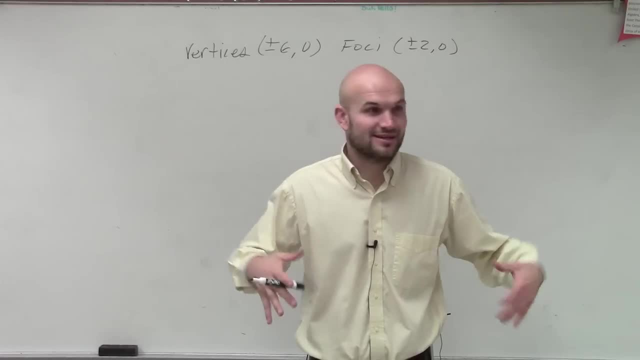 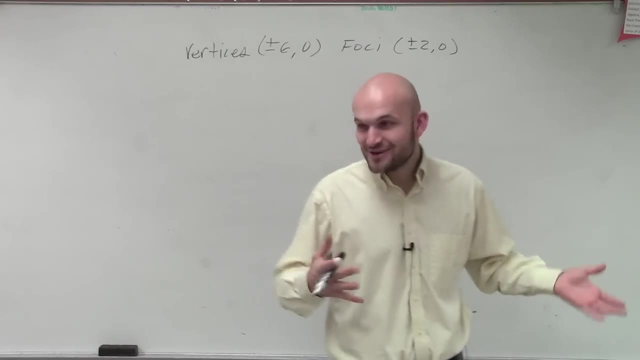 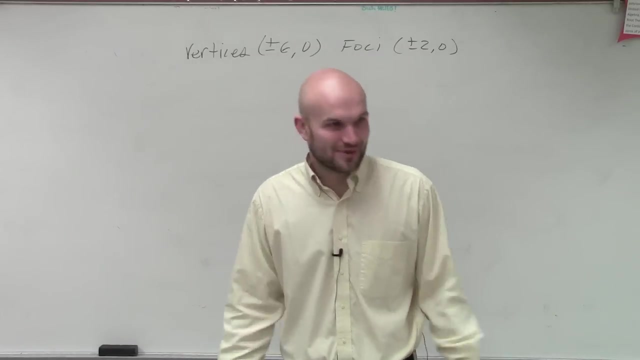 It was their early like pregnancy. So it was like for all the girls in the city like that, would you know that were having a baby, that I would be like their math teacher. So you know, just fresh out of college, Just fresh out of college, And they say, oh you know, do you think that would be a good fit? I'm just like sure, Classroom full of ladies, the women that are all ready to have a baby. That sounds like a good idea. Unfortunately, they didn't give me a call back so I wound up here. 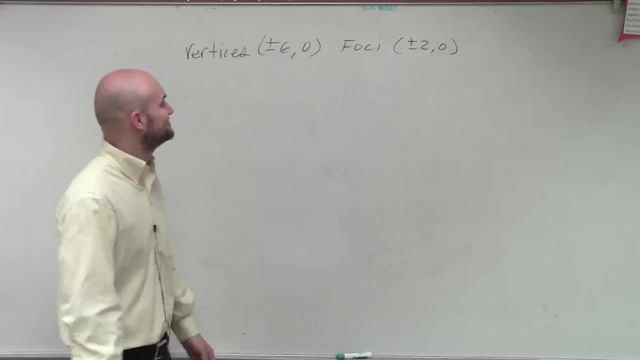 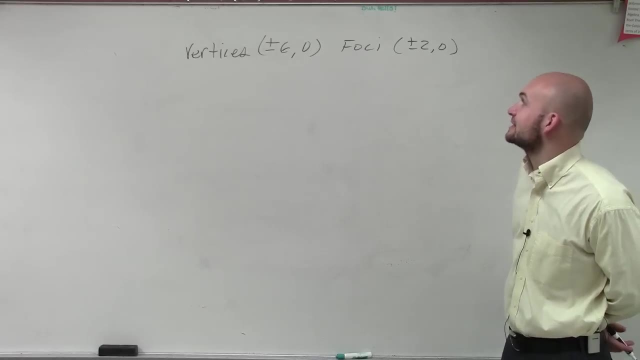 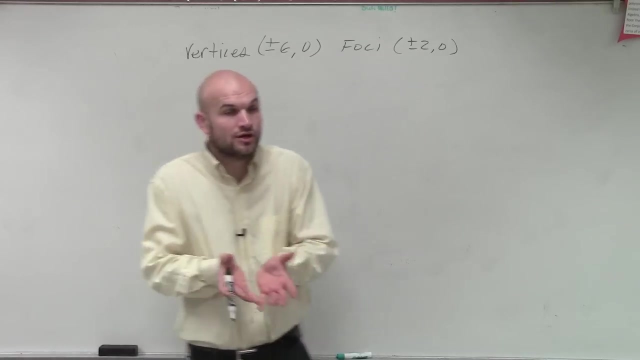 Are you guys right now? Yeah, yeah, That would be a fun intro, I guess. Anyways, so we're given the vertices negative 6, or plus or minus 6, comma 0, and the foci is plus or minus 2, comma 0. And I'm asking you to write the equation. So, ladies and gentlemen, remember the parabolas. when I said I was giving the information, The first thing I said is just there's only two equations. It's either opens up or down, or left or right right. The only way to figure that out is to plot the information and see what's going to make sense. 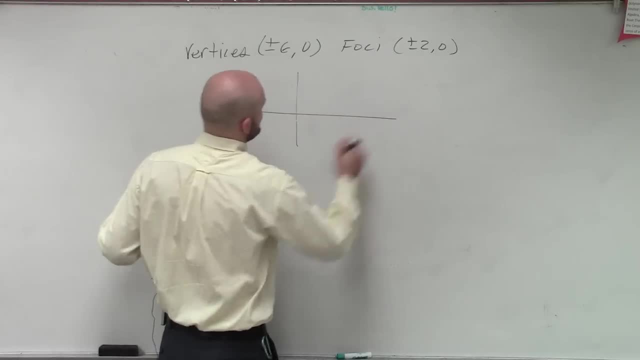 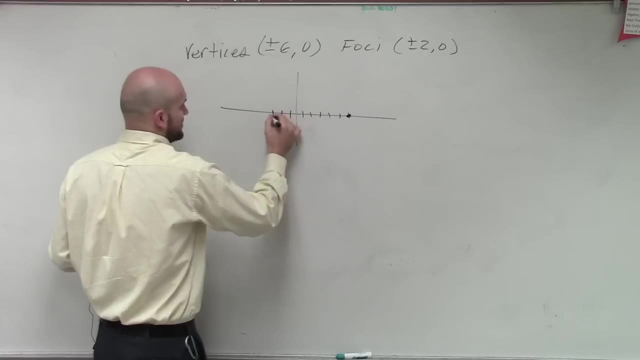 Exact same thing with this. So let's just plot the information and see what's going to make sense. So our vertices are plus or minus 6.. So 1,, 2, 3, 4, 5, 6.. 1,, 2,, 3, 4, 5, 6. Foci plus 2, negative 2.. So we have foci, foci, vertice, vertice. 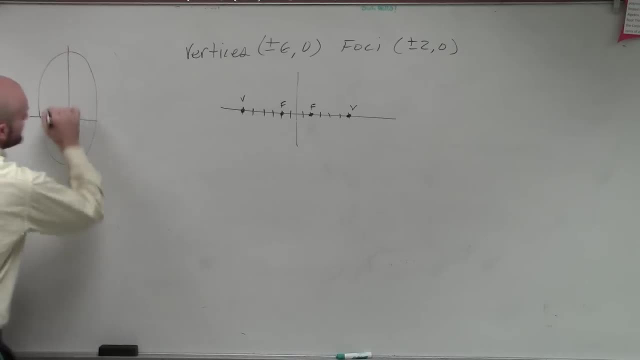 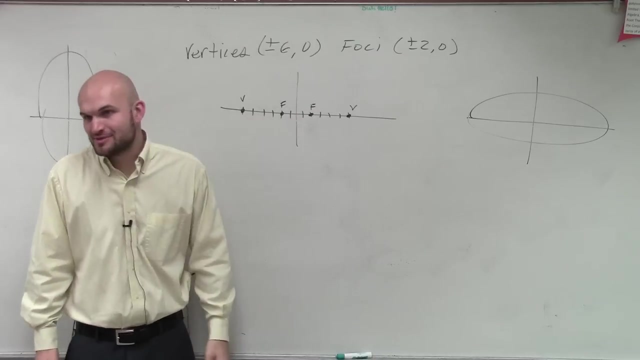 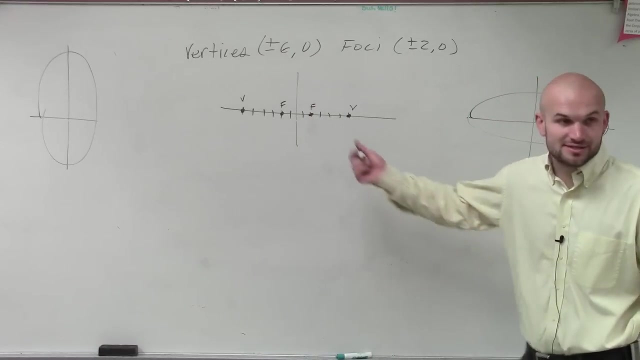 Now remember, ladies and gentlemen, there's only two ellipses that we're dealing with, One that's vertical and one that's horizontal. Now, just out of out of now, a random guess. So this is a. these are the points of one of these ellipses. Do you, would you recognize that it to be a ellipse where your major axis is vertical or where your major axis is horizontal? 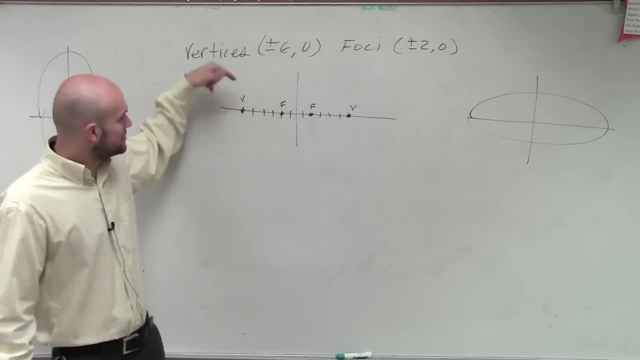 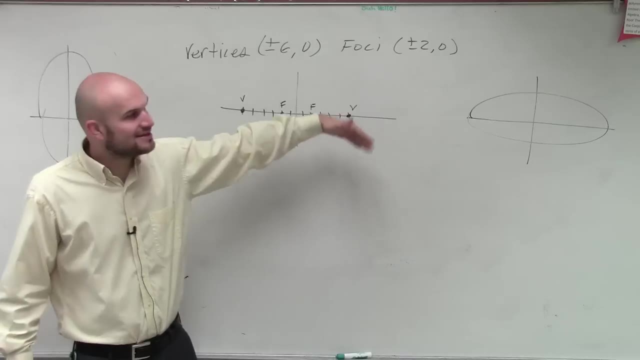 Horizontal right. It's pretty obvious. You can notice that. you know that the vertices, the foci, all have to be on the major axis And since this major axis is going horizontally, then you have a horizontal ellipse right. 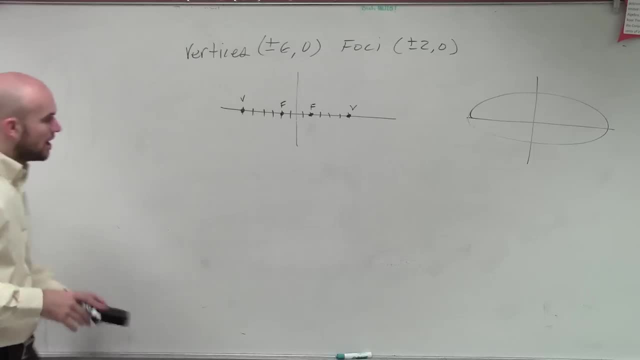 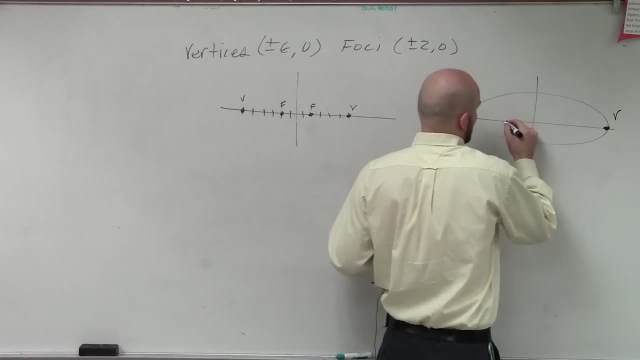 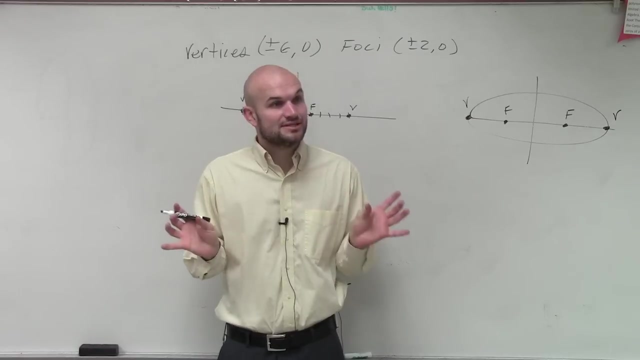 So let's just eliminate this right here. All right. Now remember when we're looking at this: if I give you the vertices and the foci, remember the vertices and the foci are plus or minus the same distance from your center, right? 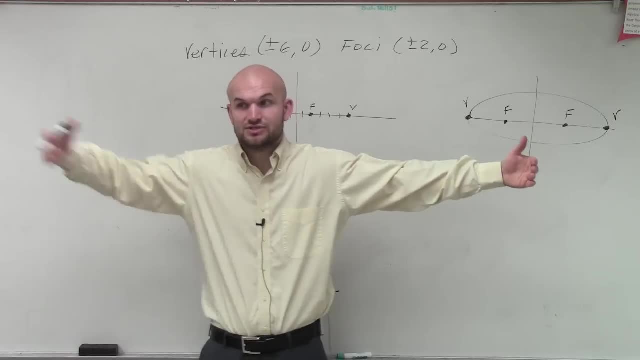 If I say your vertice is 6 units to the right, then it was also 6 units to the left, correct? So, therefore, what is going to be our center? Because we need to figure out what this center is. It's always 0, 0.. 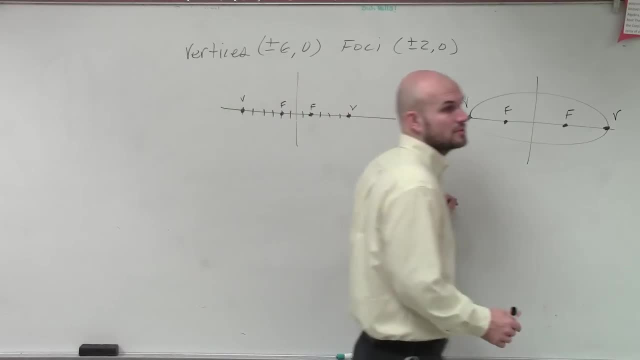 In this case, the center is 0, 0, yes, No, the Oh the problem. actually said It starts from the right. Oh, that's nice. You're right. They just say the center's at the order, So that's good. 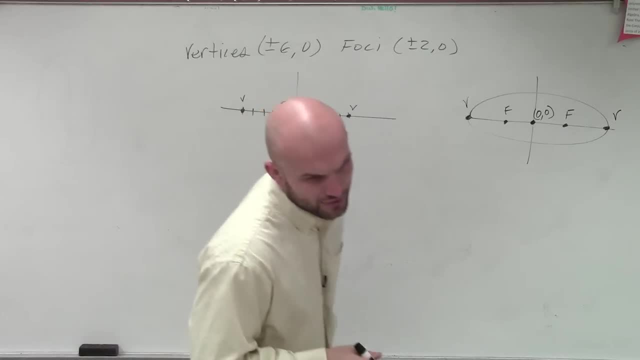 Good, Right, you're right, because all the way up to 35, then they change it to 9.. Okay, So we have, the center is 0, 0.. So that helps us, because now, when we write our equation, we know our formal was x minus h. 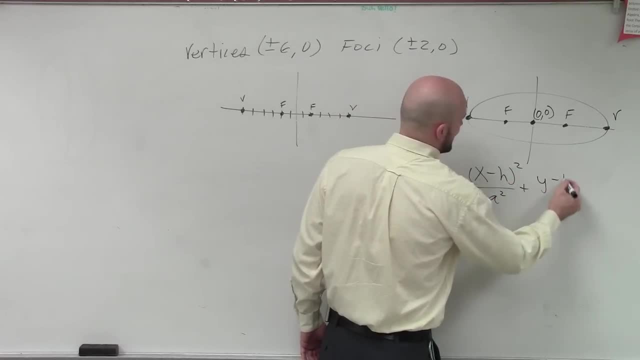 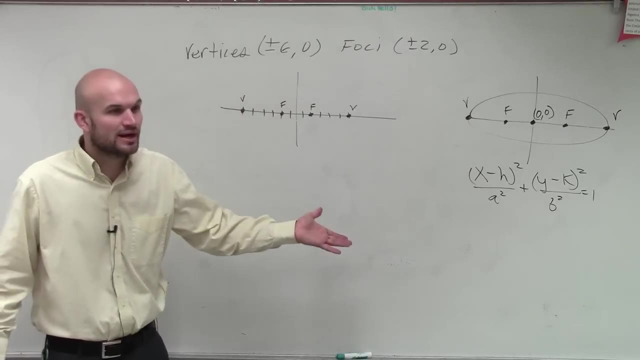 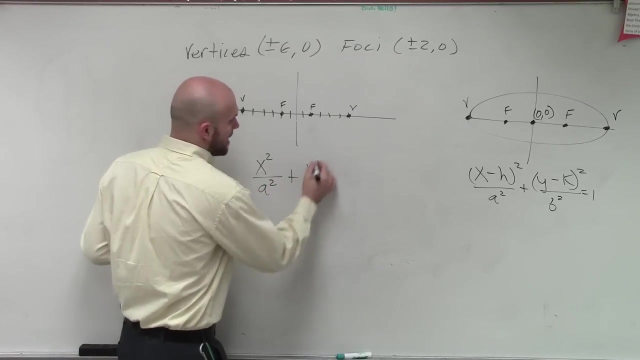 For a horizontal, then it would be: a squared plus y minus k, Squared over b, squared equals 1.. However, do we have an h and a k? Yes, there's 0, right, So now we can just say: x squared over a squared plus y squared over b, squared equals 1.. 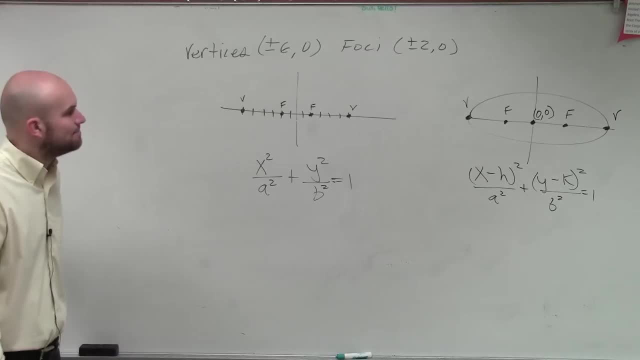 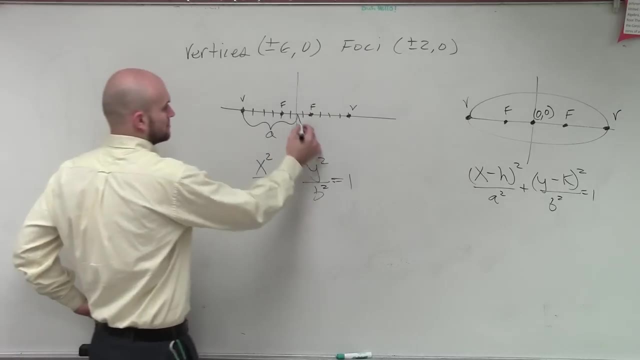 Okay, So now let's just go ahead and see if we can figure out what our a and b are. Remember, a is going to be this distance, right. It doesn't matter if it's going to be your positive or your negative. 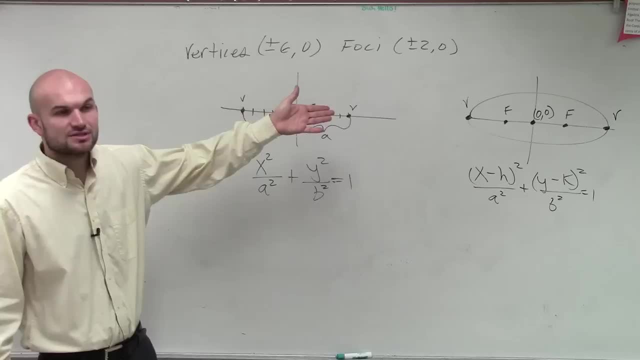 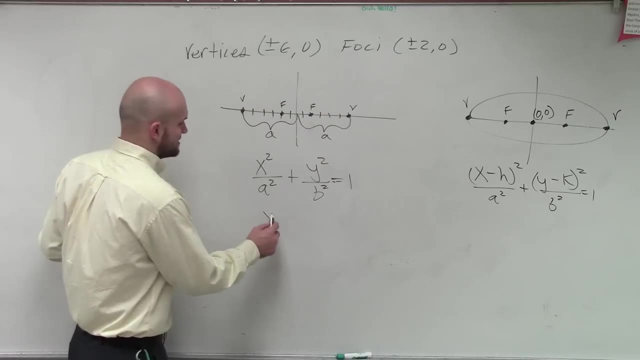 What is this distance squared? Well, the distance was 6, plus or minus 6.. You square a negative 6,. you square a positive 6. It doesn't matter, You're going to get 36. 36. Good, 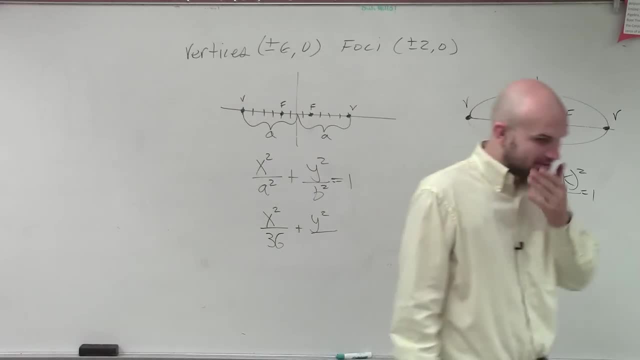 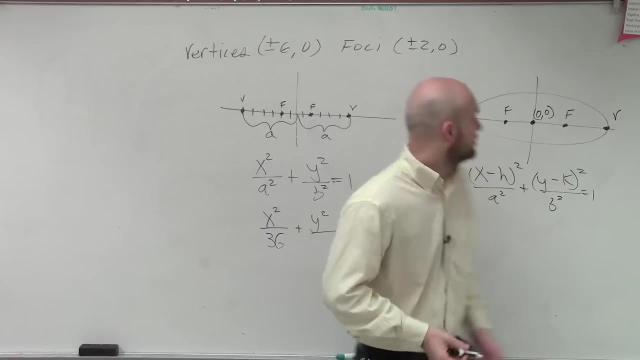 So now we have y squared over b squared. Now our problem is: we don't know what b squared is right, But the other information is we don't know what b squared is. So what we can do is we're going to use the equation that gave us was. they gave us c. 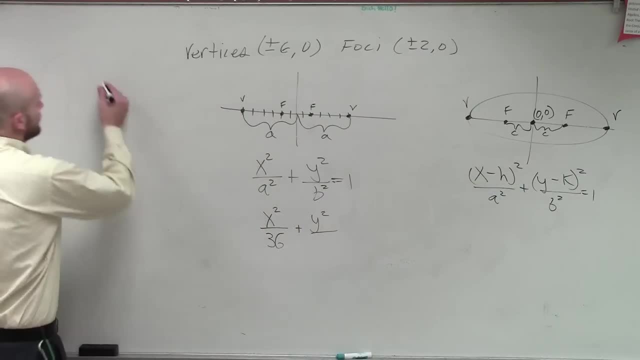 And remember we talked about a, b and c are related to each other- where we can say a squared equals b squared plus c squared. So if I know, a squared is 36 equals b squared plus c squared, so c is 2..